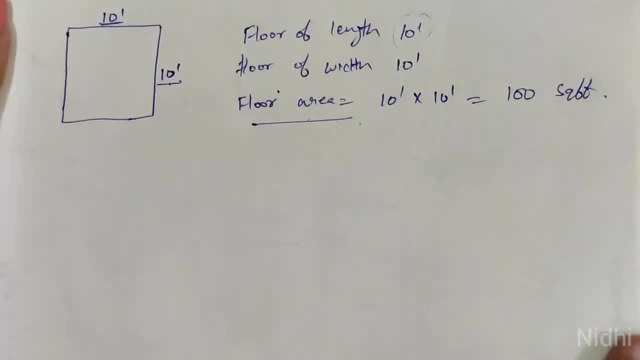 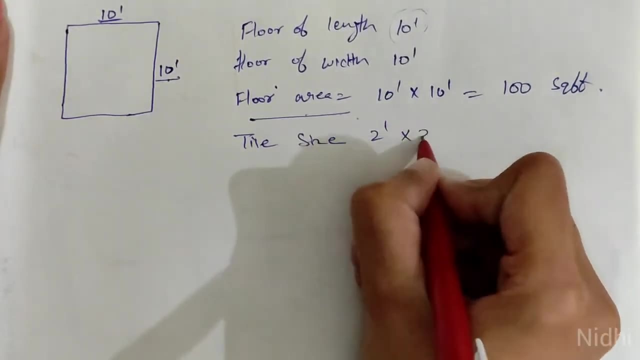 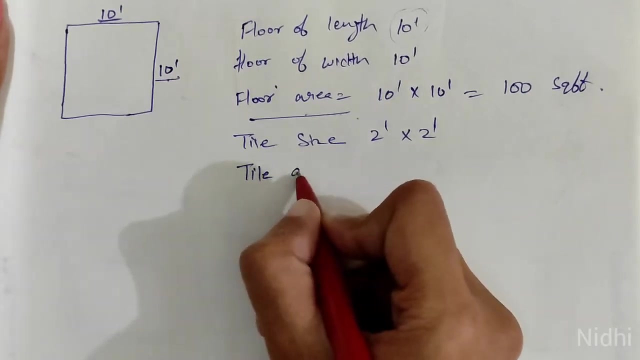 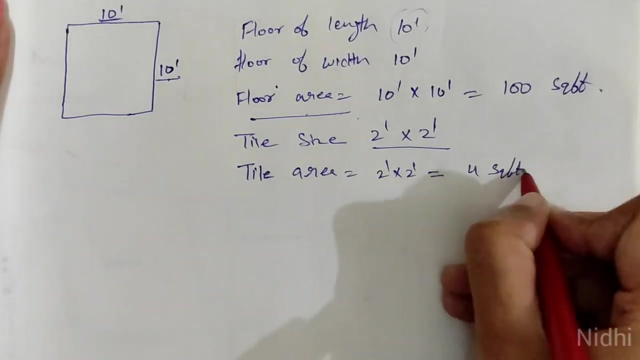 Floor area. So here we have a tile size that is 2 feet by 2 feet. So tile area, Again, 2 feet by 2 feet, is equal to 4 square feet. 100 square feet is a room area. 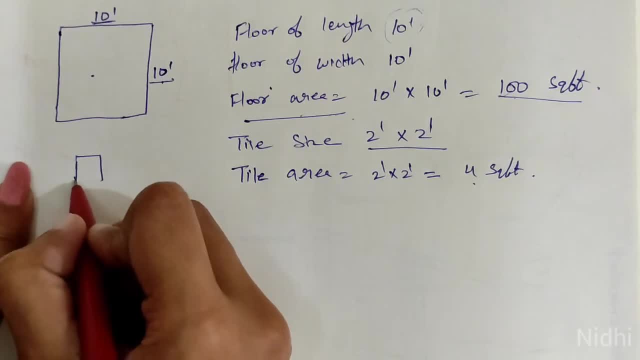 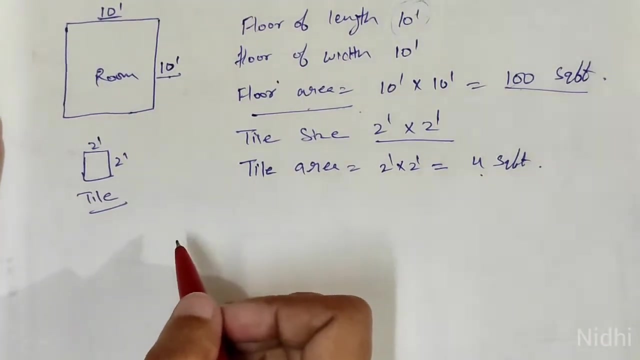 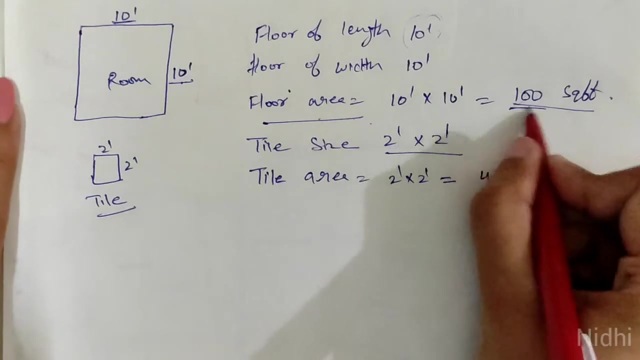 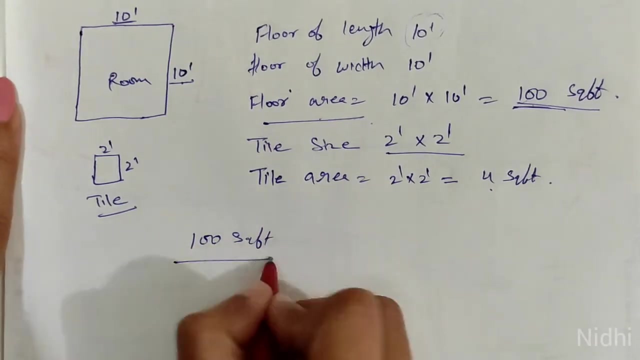 4 feet is a tile area. 4 feet is a tile area. 4 feet is a tile area. It is room And this one is a tile. So now let's check number of tiles. Number of tiles room area. that is 100 square feet by tile area. 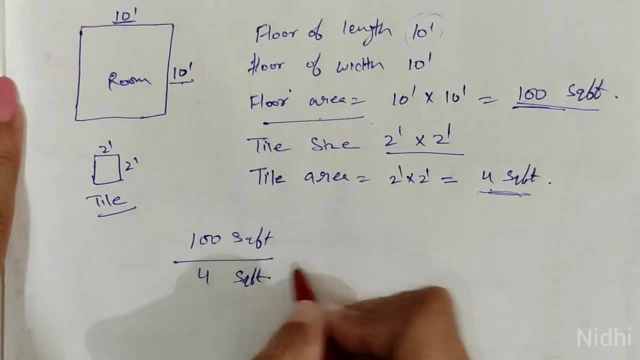 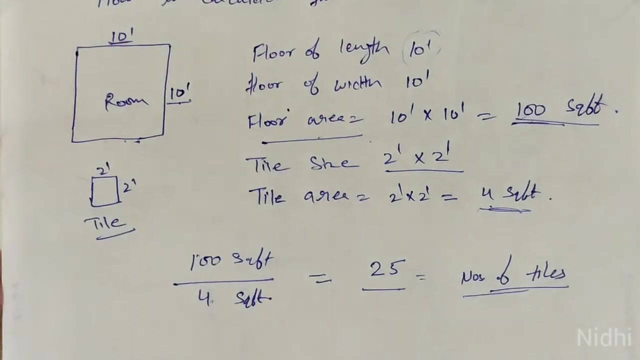 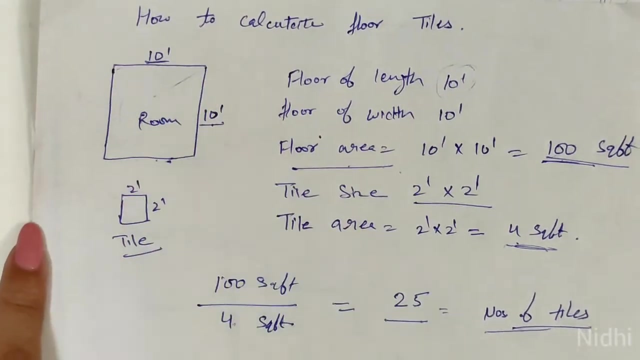 That is 4 square feet. How much will it be 25.. So this is a numbers of tiles. How many tiles will be used in this room? 25 tiles. So next, First scutting, because now we get the numbers of tiles. 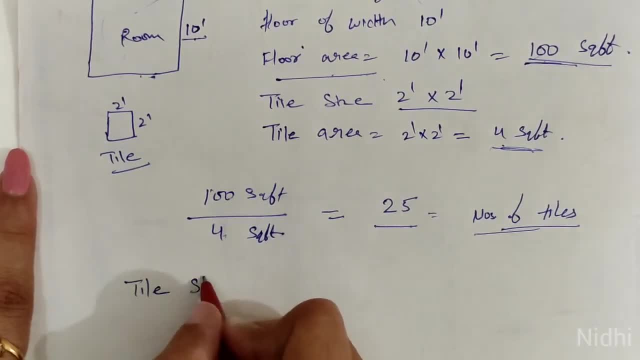 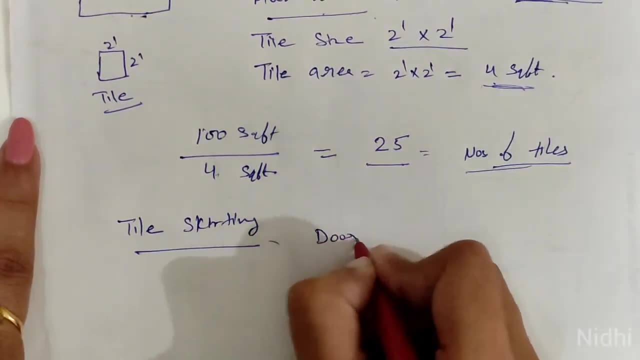 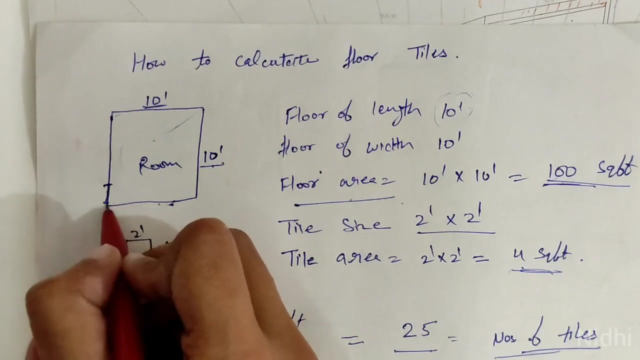 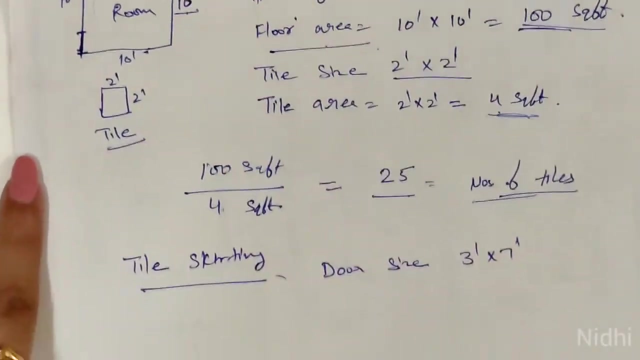 So tiles, What will we do for scutting First door size 3 feet by 7 feet, For example. door is here. Okay, 10 feet, 10 feet, It is from every side Scutting length. 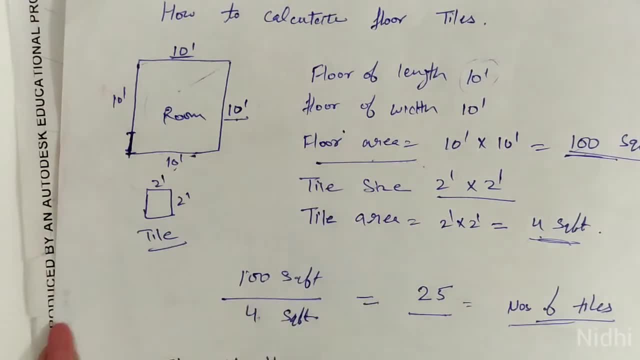 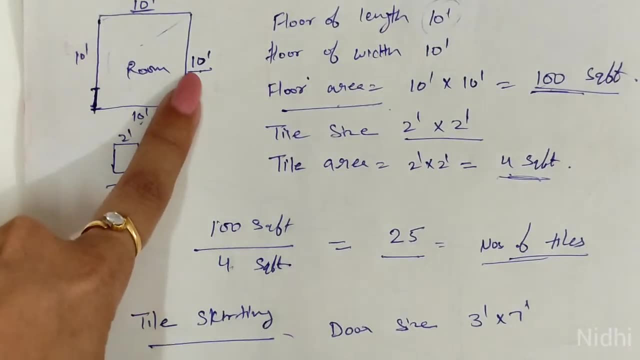 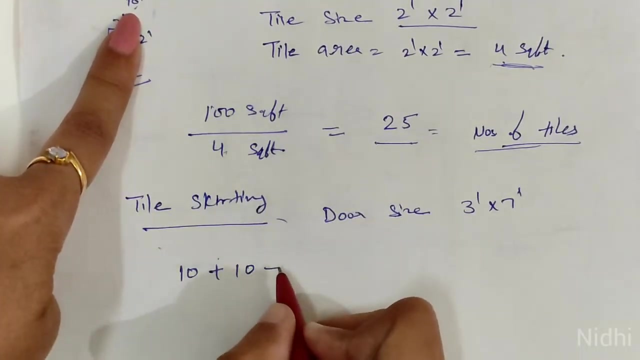 What will we do for this? Just add the all numbers First, 10., Okay, 10.. And again this plus the sign: Again, 10.. This one Again, plus 10.. Here, what is 3 feet? This is a door. 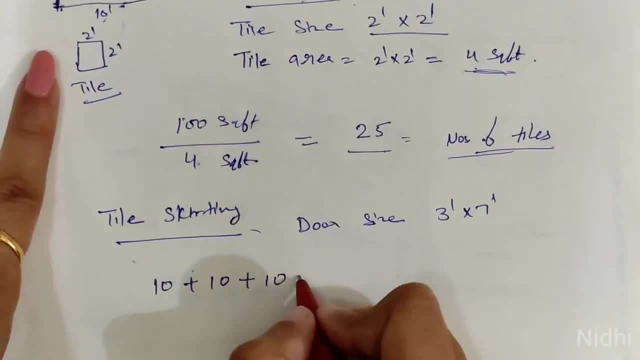 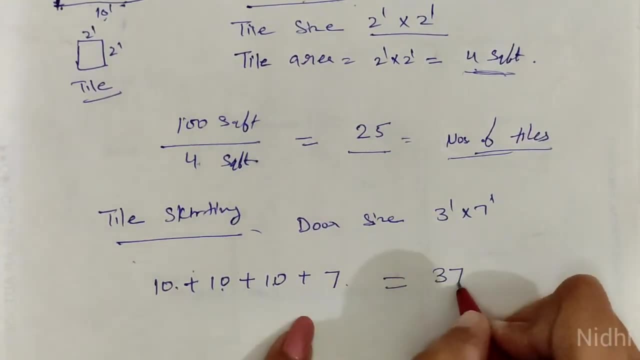 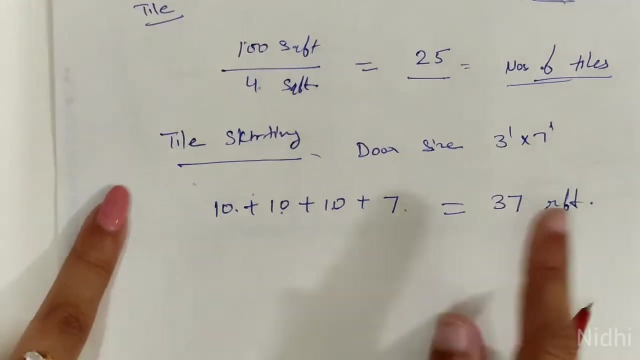 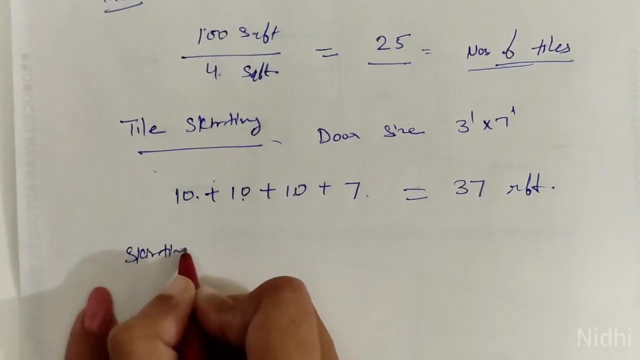 So 10 minus 3. Here we have a 7. 10 plus 10 plus 10 plus 7. That is 37. Running feet. So scutting area, Scutting area, This is length, This is length. 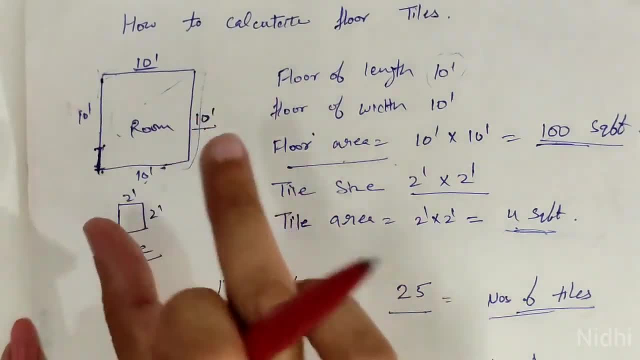 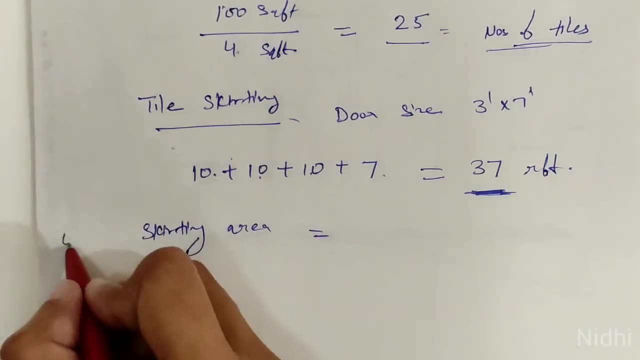 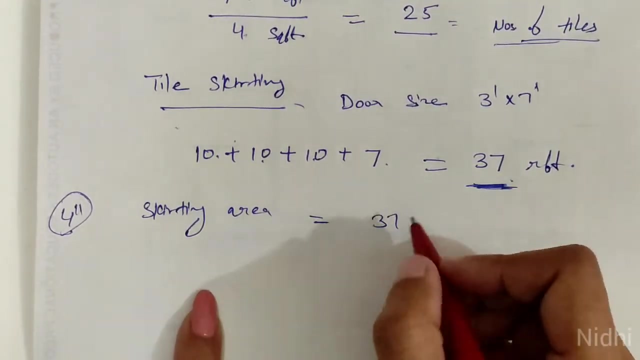 We have only calculated this. So the height of the scutting: Here we are using 4 inches. Okay, 4 inches Scutting height. For that you have to do 37. This one, 37. Here you have to write. 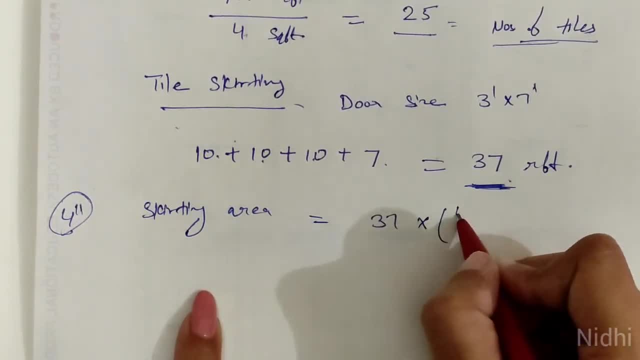 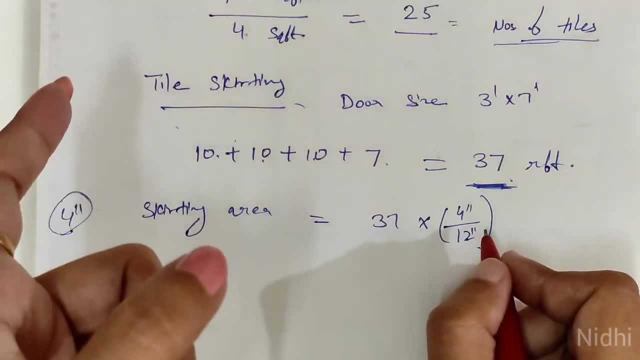 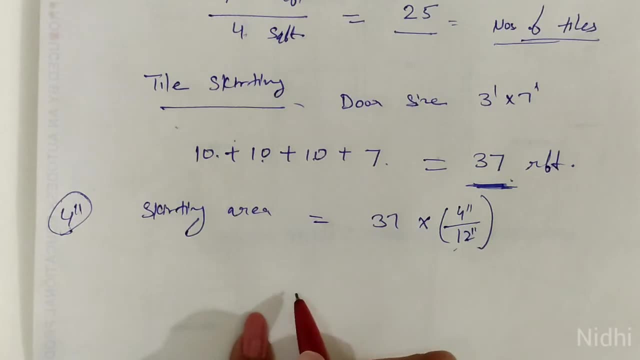 Okay, Because this is a 1 feet. 12 inches is a 1 feet, So here we are using that 12 inches. The answer which we have will be that is 12.33.. This is our running feet area for scutting. 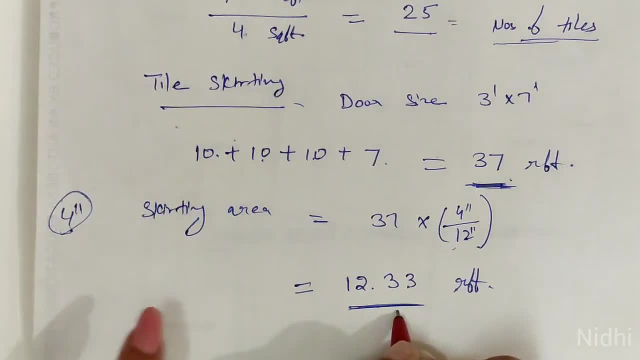 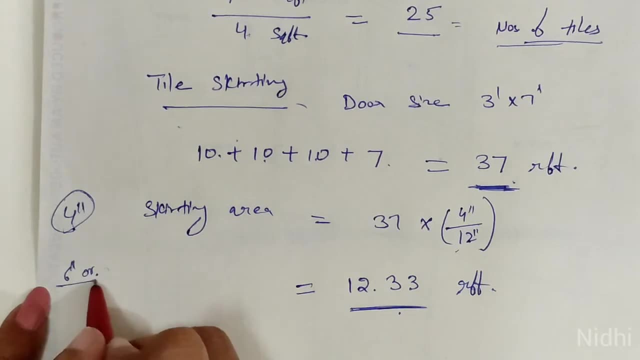 Always, we are using running feet where we have a 6 inches. 6 inches Same as r r. 1 inches Same as r,1. Same as ri. where ever you have to calculate it, we will use running feet. 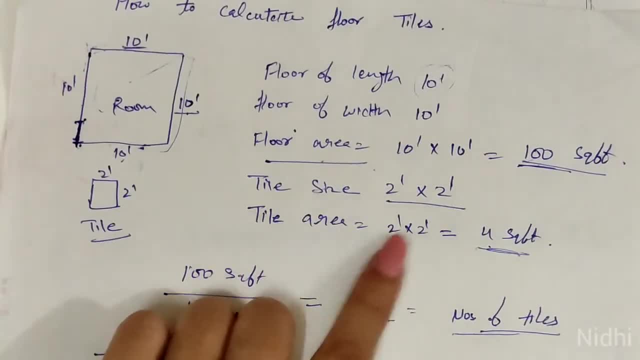 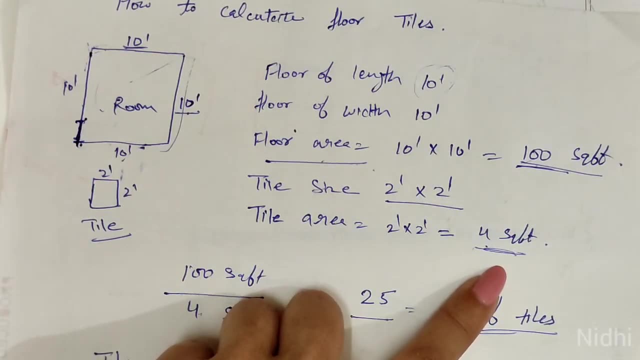 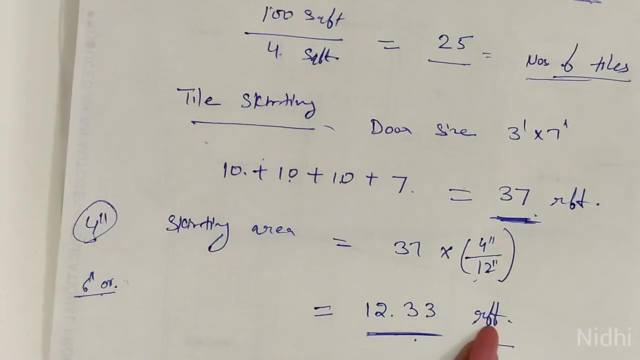 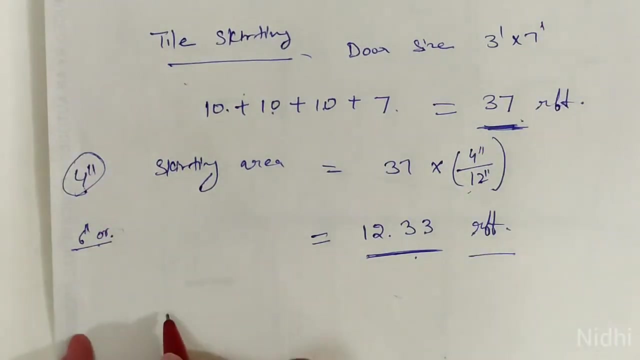 here we have 2 feet by 2 feet area and 10 feet by 10 feet area, so we used this thing in square feet. where ever you have less than 6 feet area, we will use it in running feet. so total area will be room. total area we have 100.